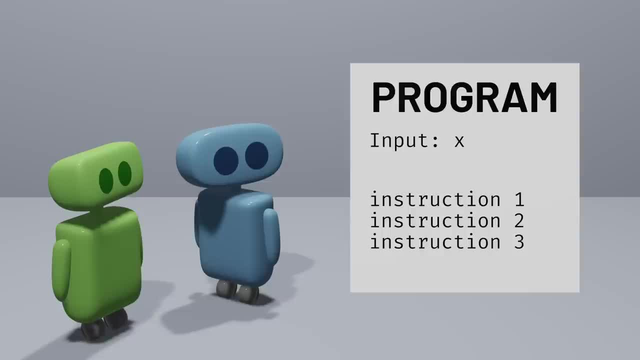 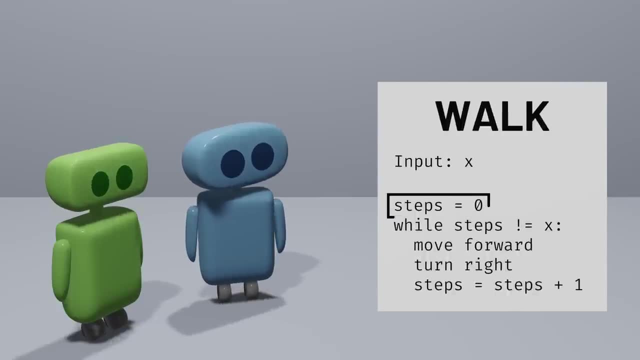 inputs so that the program behaves differently depending on what input is provided to the program. Here, for example, is a program called walk that starts by keeping track of a variable steps which starts out as 0. As long as the steps value isn't equal to the input to the program, the program instructs us. 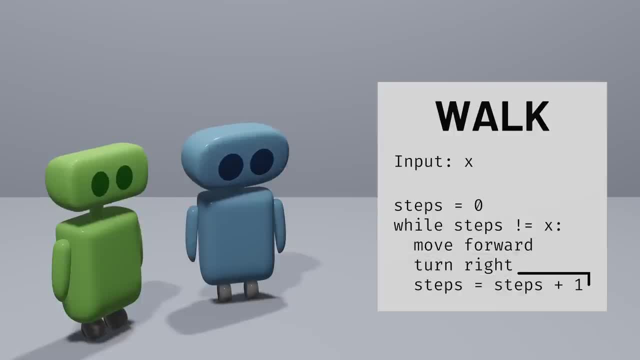 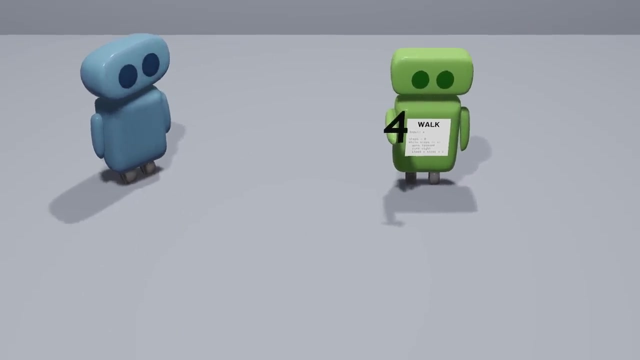 to move forward, turn right and then increase steps by 1. That keeps repeating until steps is equal to the input, at which point the program terminates. If we give this program to a computer and then give it an input like the number 4, then the computer will repeat the process four times. 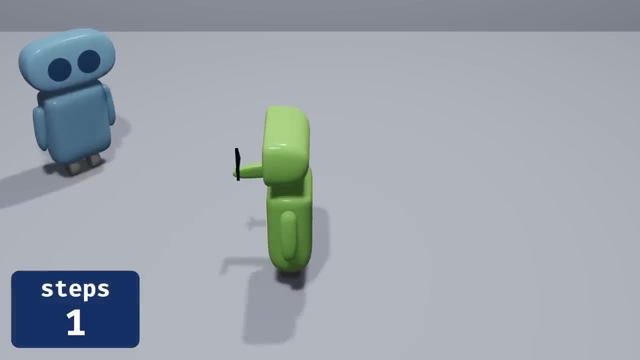 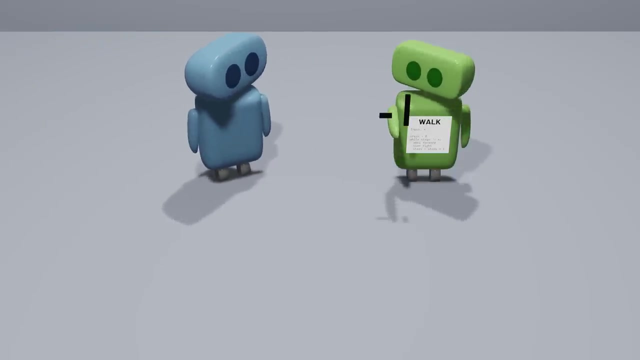 Moving, turning, increasing its internal step counter And after repeating four times, the program terminates. In other words, when the program is done running all of its instructions, it will halt. But if we give the same program a different input, like the number negative 1,. 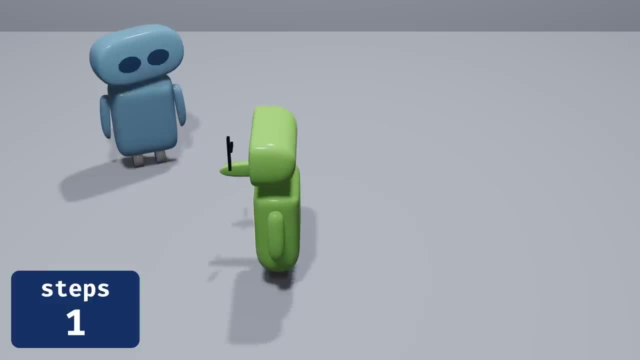 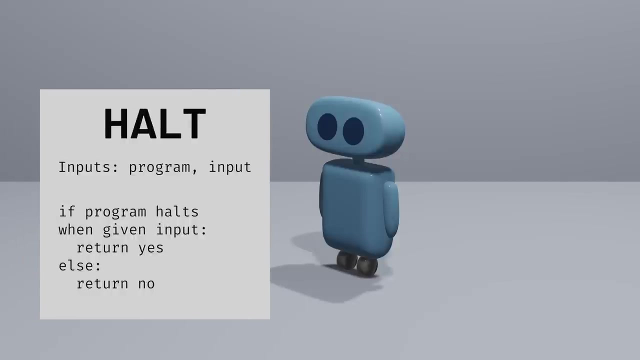 the computer will keep running this program forever. Every time the loop runs, the step counter increases by one, but the counter will never reach negative 1, so with this input the program will never circuit, never halt. So here's our question: Could we define a new program halt that accepts a program? 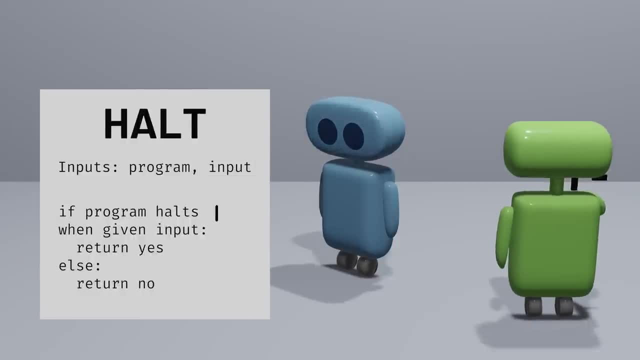 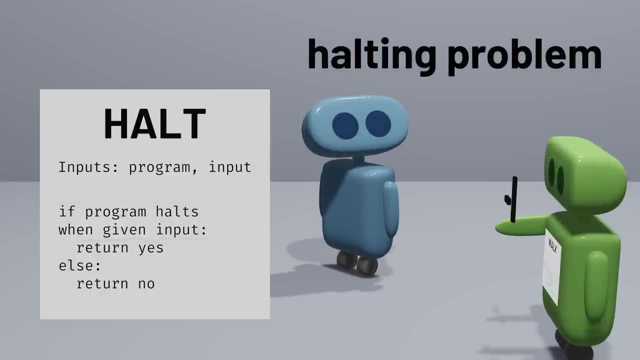 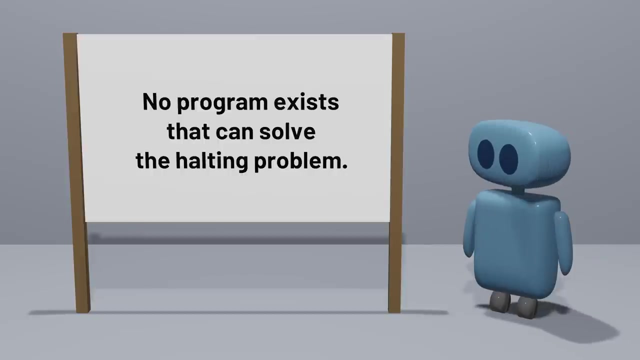 and an input and tells us whether that program will halt when run on that input. This is the halting problem, and it's a famous problem in computer science. The answer, it turns out, is that the halting problem can't be solved. Not only is there no program that exists that can. 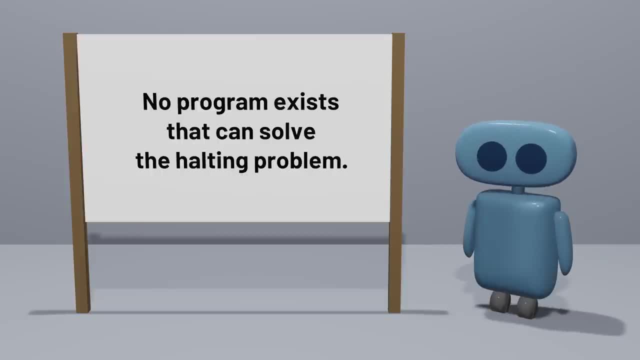 solve the halting problem. but we can actually prove that there could never be a program that solves the halting problem. So let's prove it. Let's prove that the halting problem can't be solved. We'll approach this proof using a common technique known as proof by contradiction. We're 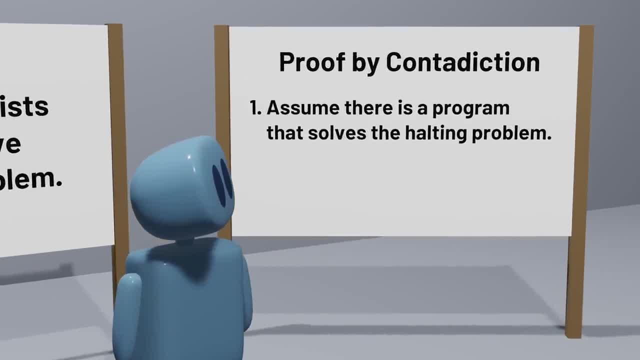 going to start by assuming that there is a program that solves the halting problem and show that if such a program were to exist, it would lead to a contradiction, some situation that logically doesn't make sense and couldn't possibly be true. Let's give it a try. Say we had some program. 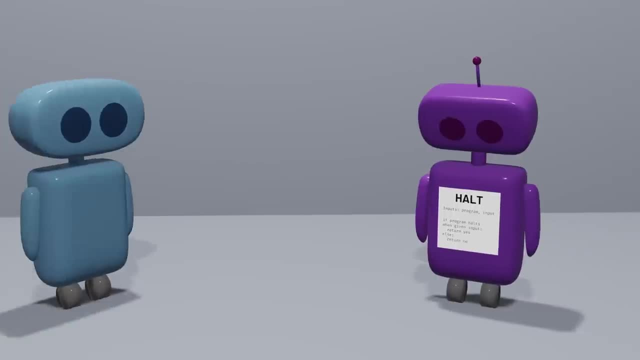 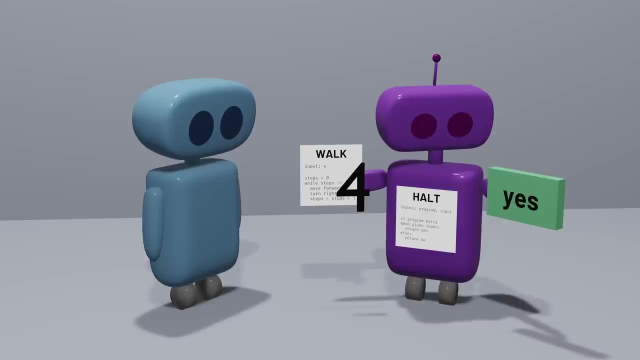 called halt that could solve the halting problem. Let's say that there was a program called halting problem. It could take a program and an input, perform some computation and then give us back an answer: Either yes, the program does halt on the input or no, the program does not halt on. 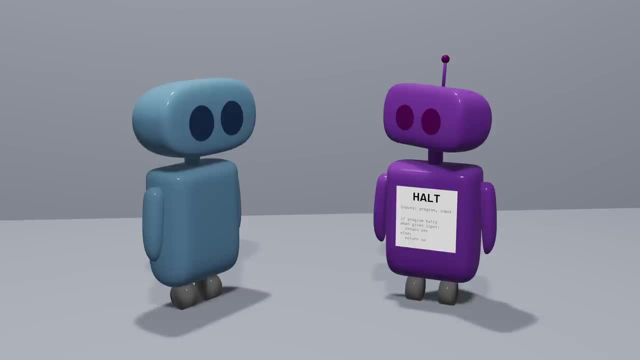 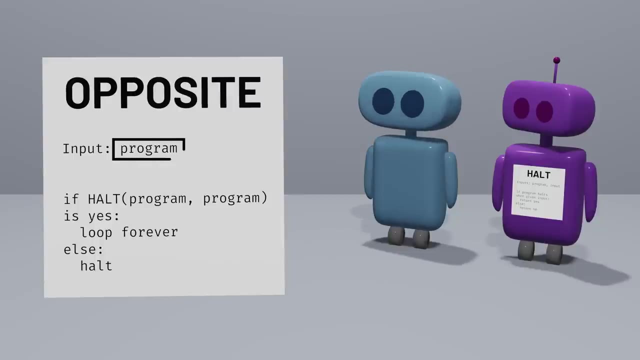 the input. If such a program were to exist, we could then use it inside of other programs. Here, for example, is a program called opposite. It accepts an input program and then uses the halt program to see whether the input program will halt when given the input program itself. 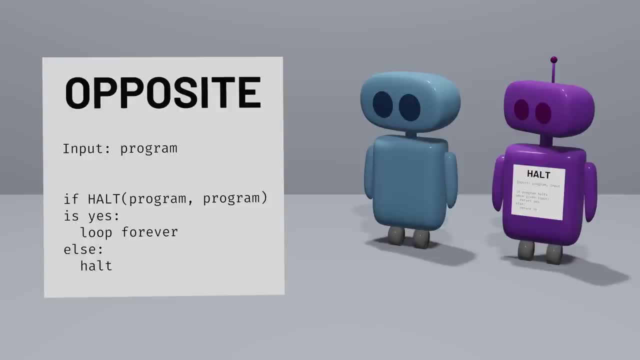 as its input. The reason we've called this larger program opposite is because whatever halt tells us, we're going to do the opposite. If halt says yes, the program will halt, then opposite will do the opposite and never halt as by looping forever. If halt says no, the program won't halt, then 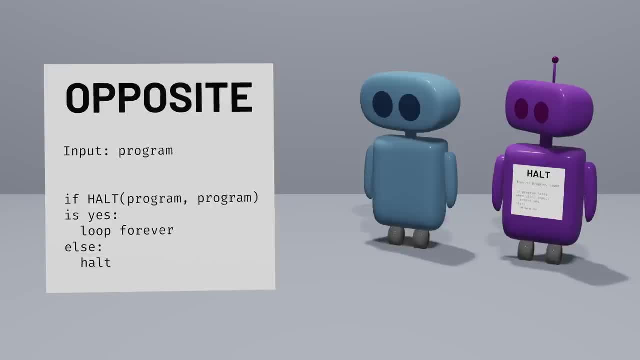 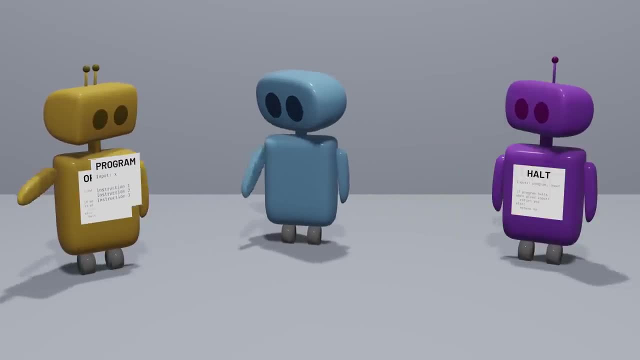 opposite will terminate and halt the running of the program. So if we have a computer run this opposite program, it'll work like this: We give the program some input, the computer will take the input and pass it along to the halt program, checking to see whether that program 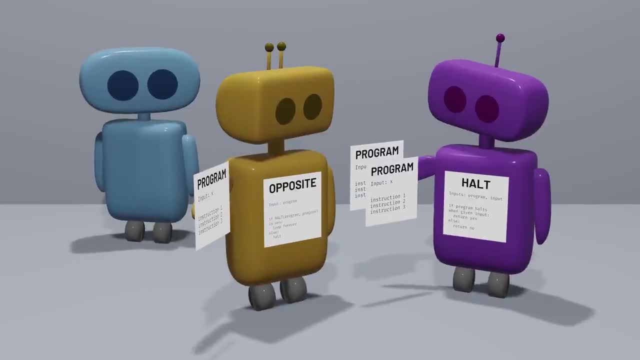 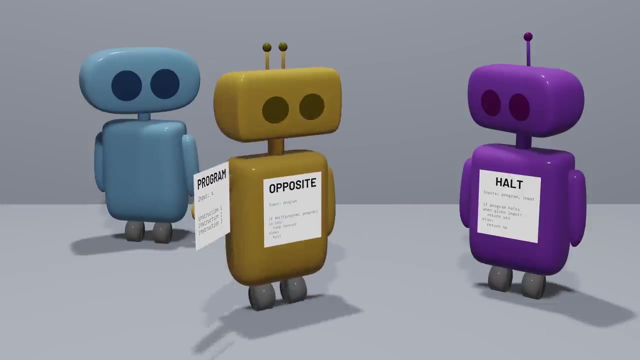 will halt when given itself as input. Whatever halt says opposite does the opposite. If halt says the input program halts, then opposite will do the opposite and loop forever, never halting. Importantly, as long as it's possible to write the halt program, it's also possible to write: 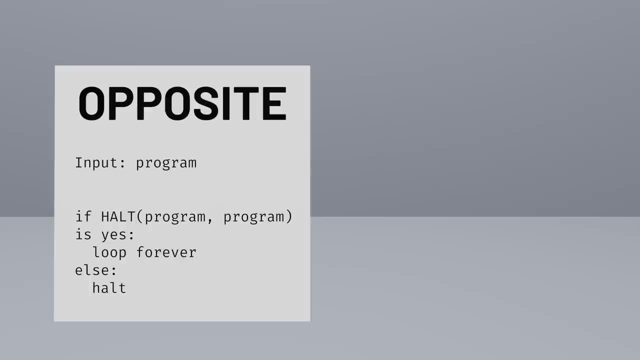 this opposite program, since we're just adding some logic like conditional constructs and looping. So if we have a computer run this opposite program, we're going to do the opposite that we know computer programs can use. But now here's the tricky question: What happens if we use? 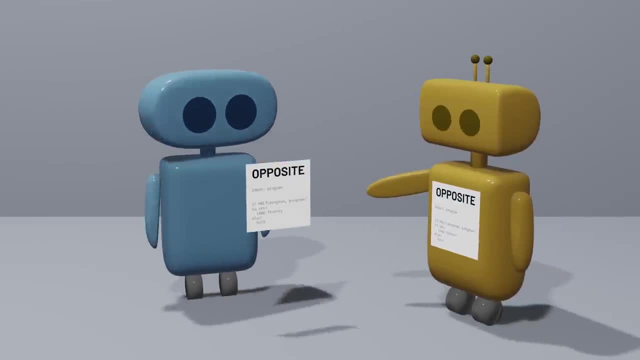 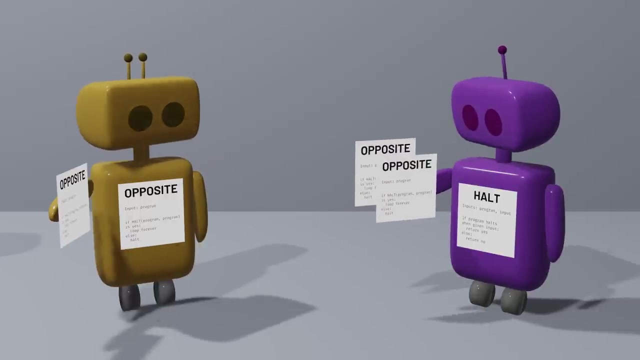 the opposite program itself as the input to the opposite program, Does the program halt? Well, let's consider what might happen. Following the program's instructions, the first thing that happens is that we ask the halt program whether the opposite program will halt when given the opposite program as input. There are two possibilities, Possibilities. 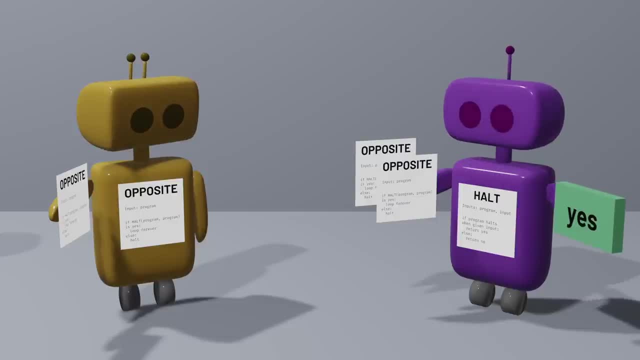 one is that halt says yes, the opposite program will halt when given the opposite program as input, Then our program does the opposite and decides not to halt. But that doesn't make sense because halt said that the program would halt in this case. Possibility two is that halt says no. 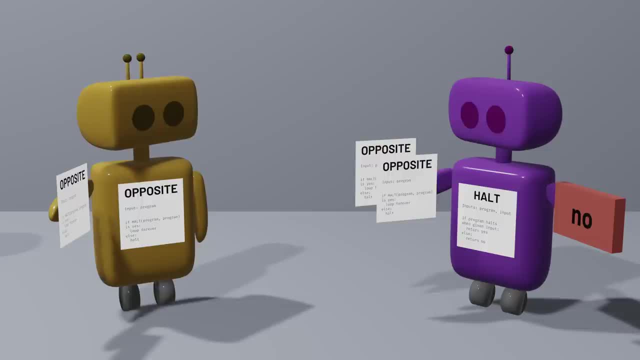 the opposite program will not halt when given the opposite program as input, Then our program does the opposite and decides to halt Again. this doesn't make sense because halt said, our program wouldn't halt in this case. Either way, we've reached a contradiction.